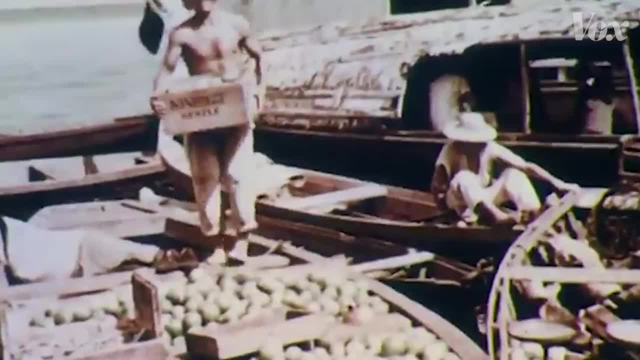 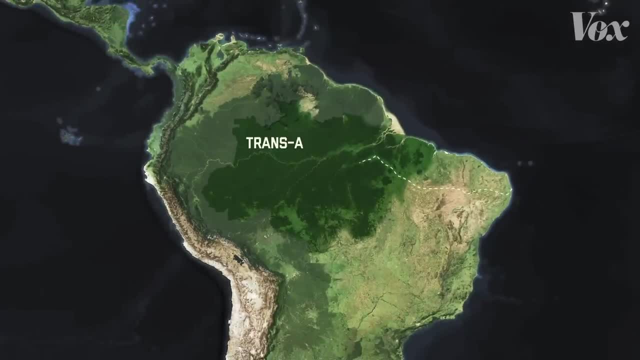 Amazonia's ores and minerals, food, fiber and forest resources are vast, But most of it was inaccessible. So the government started building the Trans-Amazonian Highway, an ambitious project that would run for 3,200 kilometers, connecting remote parts of the rainforest. 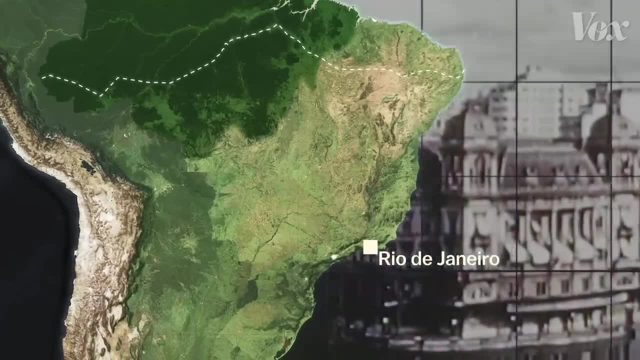 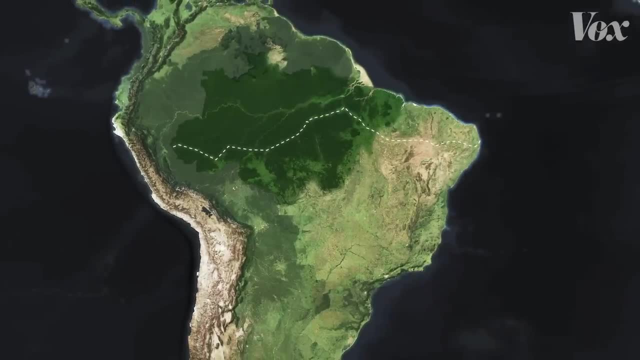 At the time, most of Brazil's population lived in the southeast, in cities like Rio de Janeiro and São Paulo, And the government wanted to move people out here to cultivate the land and grow the economy, So they offered free land along the highway. 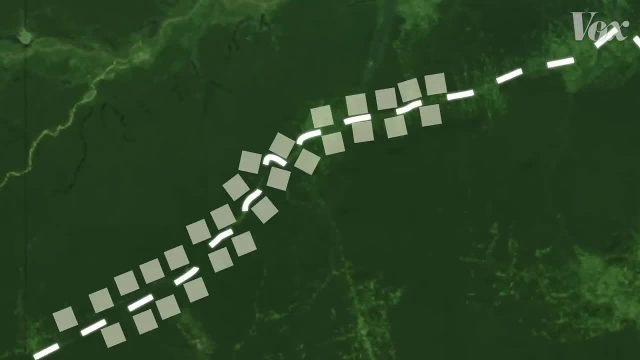 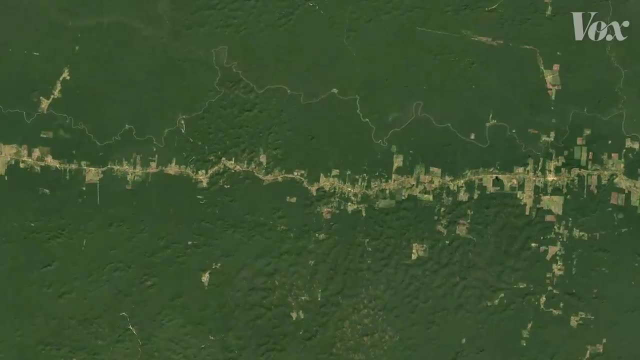 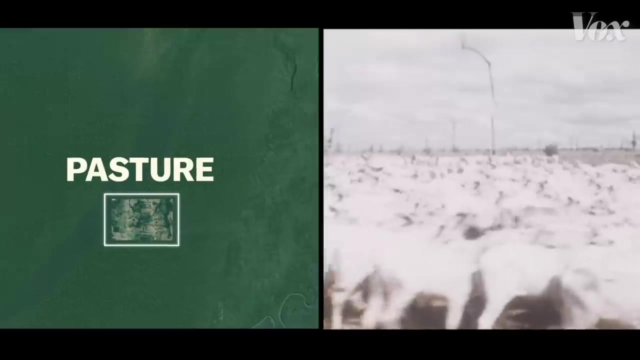 and paid Brazilians to settle deeper in the rainforest, And they sparked a land rush. As the roads advanced, settlers followed, rapidly clearing the forest around it. Most of them turned their land into pasture where they raised cows to sell as beef. 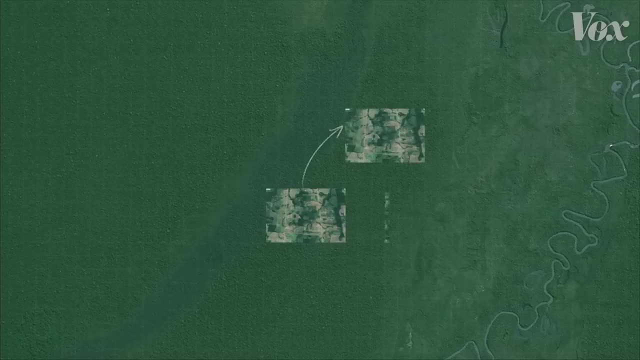 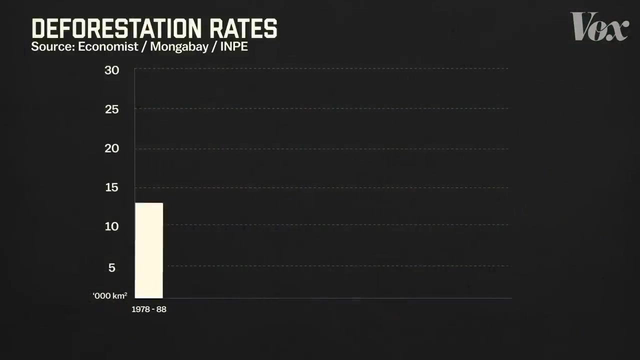 And when these ranchers needed more land, they seized another plot, cleared it and moved their cattle. in This expansion deeper into the Amazon drove up deforestation. Between 1978 and 88, an average of over 20,000 square kilometers were cut down each year. 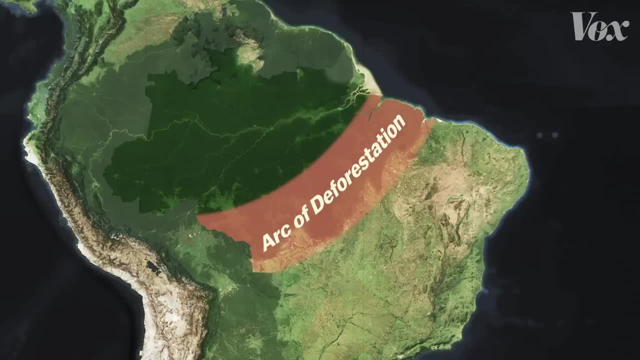 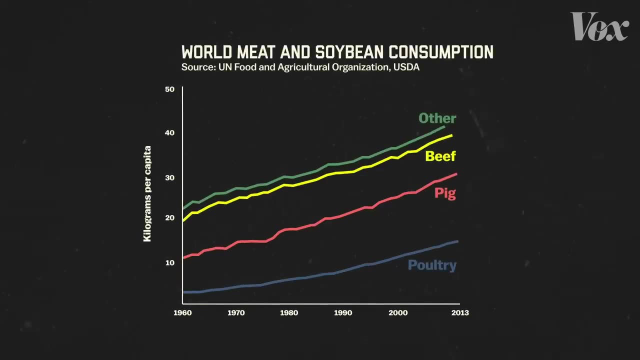 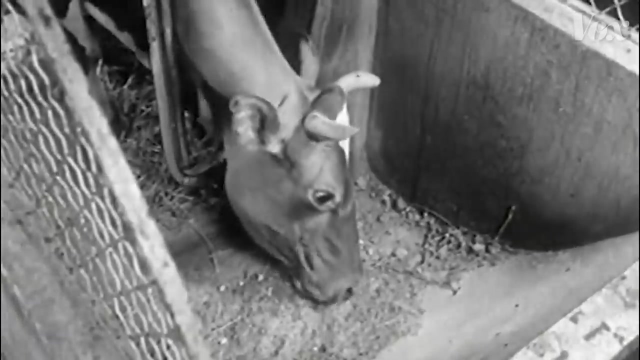 Over time, this whole area became known as the Arg of Deforestation, And soon a different product pushed this even further. People around the world were eating more meat. decade after decade, That trend raised the need for more soybeans, which served as a high-protein feed for farmed animals. 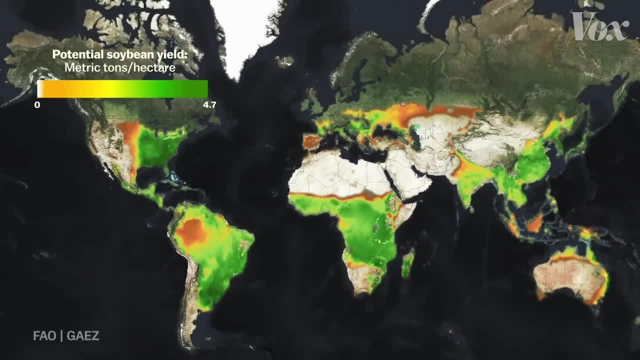 This created a demand for more soybeans which served as a high-protein feed for farmed animals. This created a demand for more soybeans which served as a high-protein feed for farmed animals. This created a huge opportunity for countries most suitable for growing soybeans. 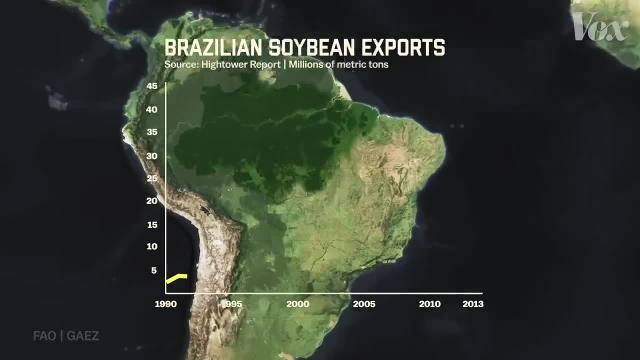 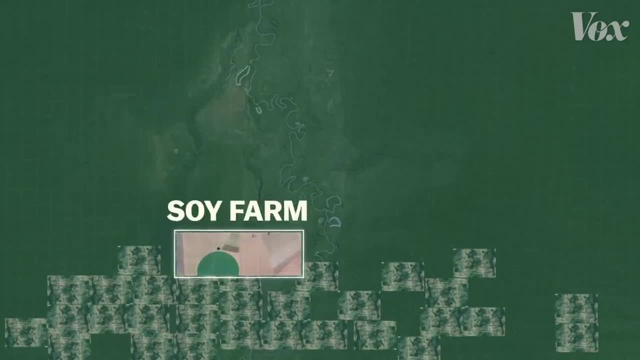 and Brazil cashed in. Soybean exports from Brazil shot up in the mid-90s, boosting the economy. By the early 2000s, farmers took over these pastures and turned them into massive soy farms Like this one in Acre State. 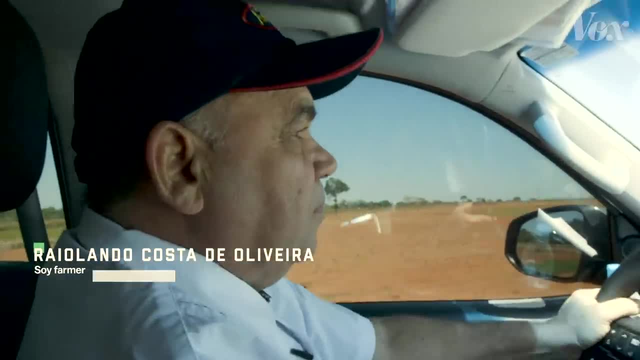 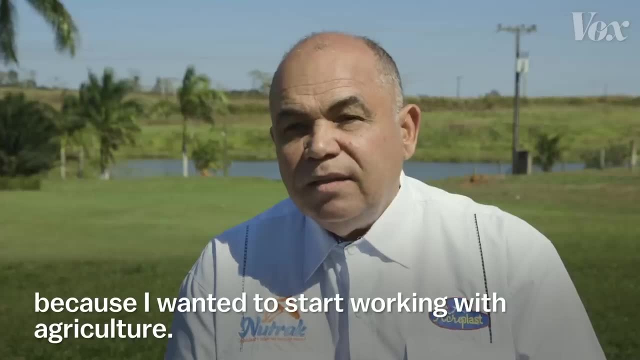 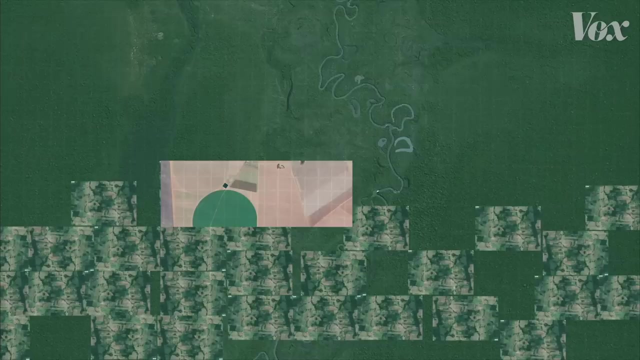 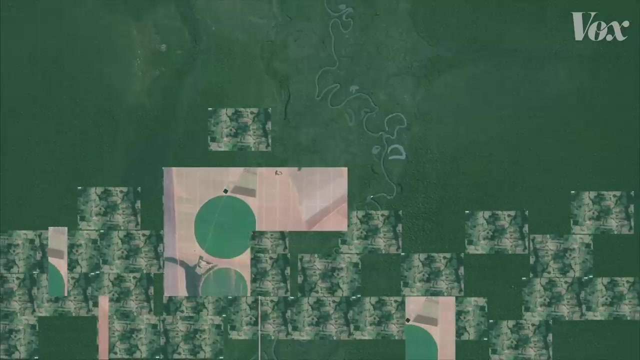 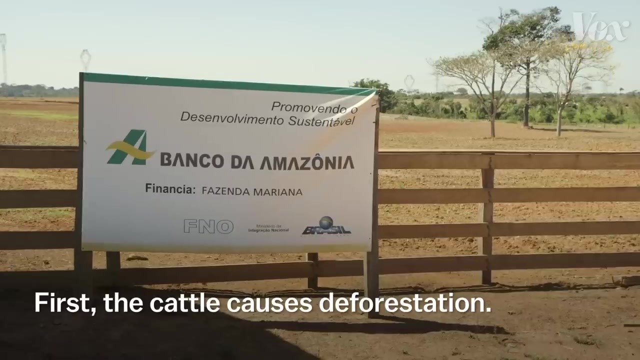 I bought my farm in 2000 because I wanted to start farming, And the ranchers who sold their pastures moved their cattle further into the rainforest, clearing more of the Amazon, often illegally. This aggressive expansion created a profitable pattern in the Amazon. 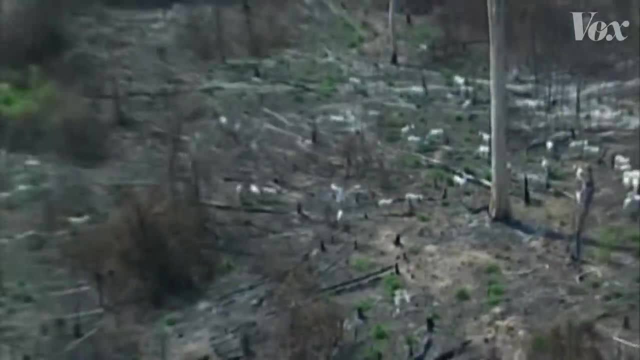 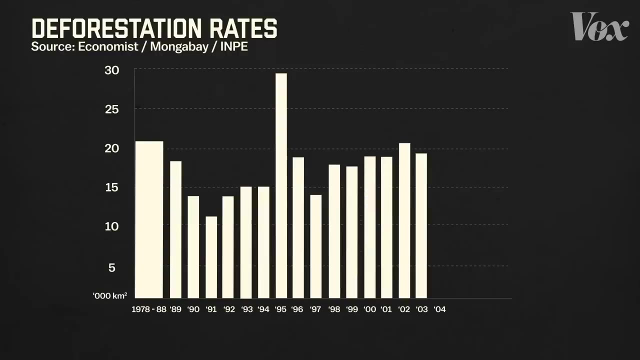 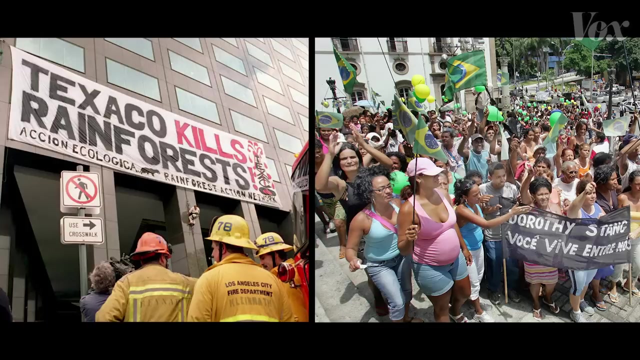 But it came at the cost of the rainforest. By the early 2000s, Brazil's beef and soy industries were driving a booming economy as well as unprecedented rates of deforestation, which caused this arc to expand further north. The staggering deforestation in the Amazon attracted fierce resistance from environmental 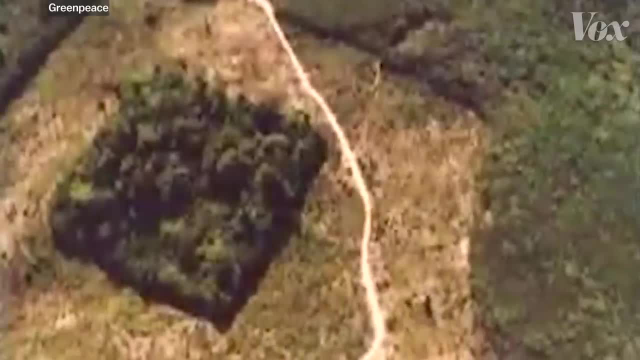 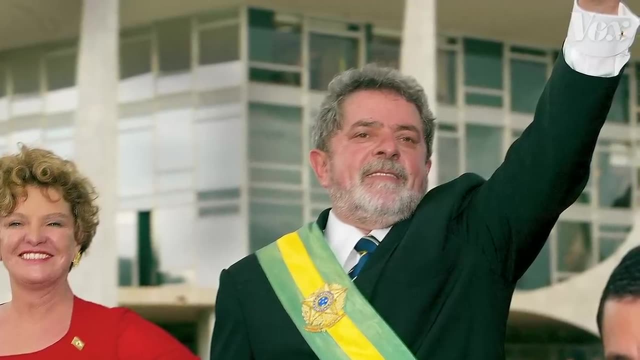 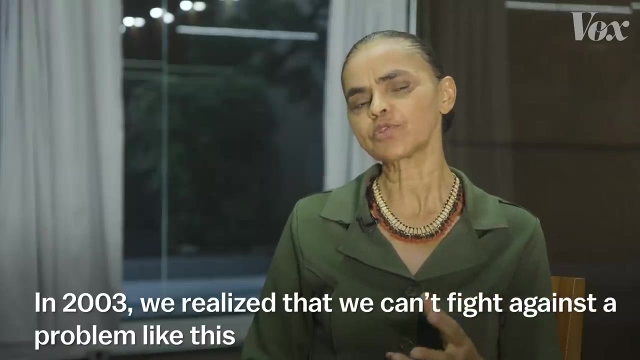 groups. An area of ancient forest the size of a football field is destroyed every two seconds. The Brazilian government under President Lula did this. Marina Silva finally stepped in In 2003,. we realized that this type of situation cannot be fought only with emergency actions. 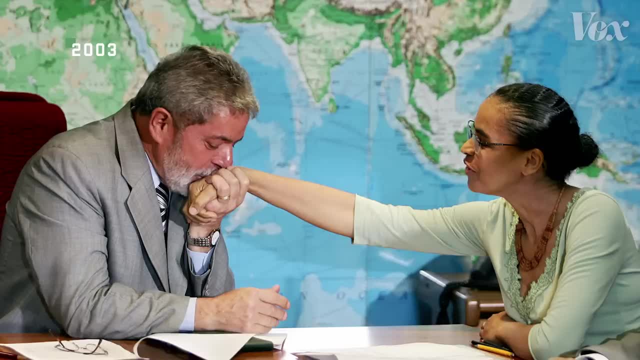 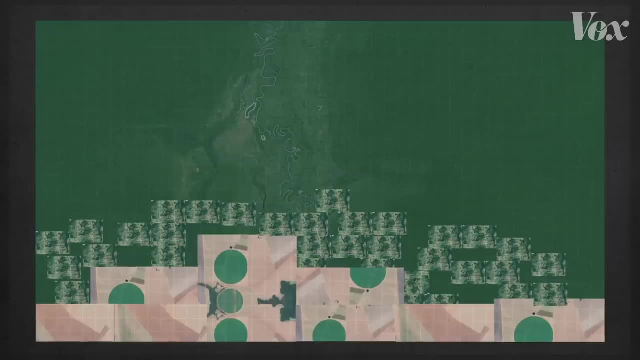 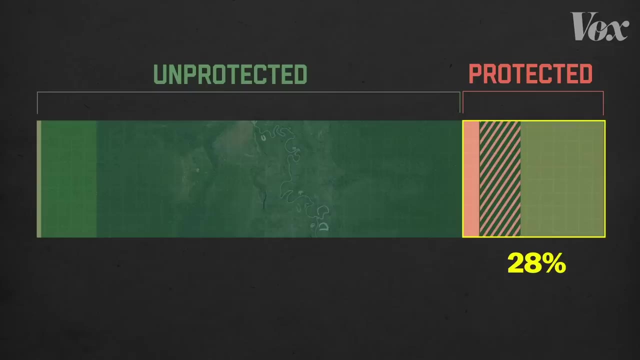 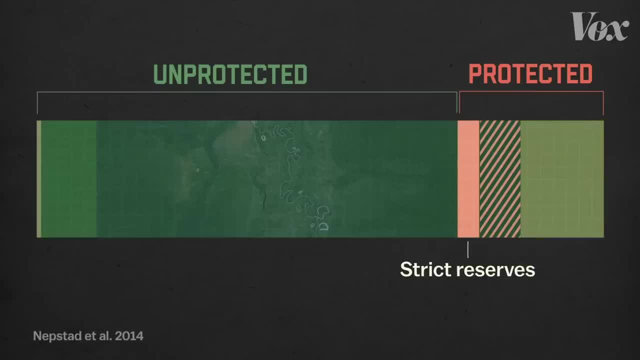 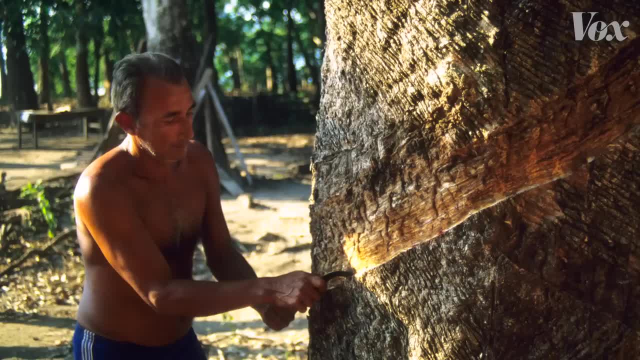 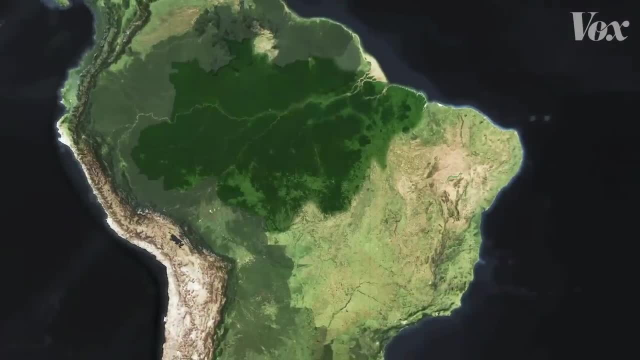 and rubber tapping, which didn't destroy the rainforest, were allowed. More land was also demarcated for indigenous people who preserved the forest. Over time, hundreds of new protected lands were added, transforming the Amazon into a shared and sustainable space. 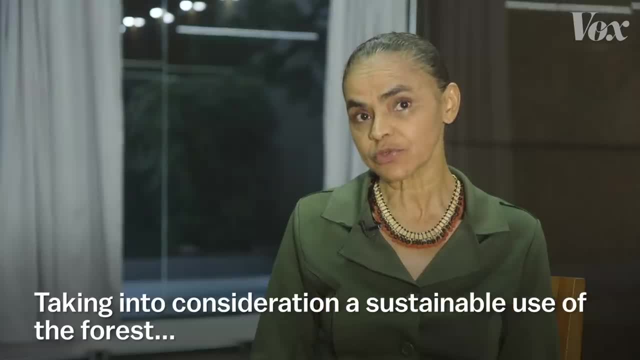 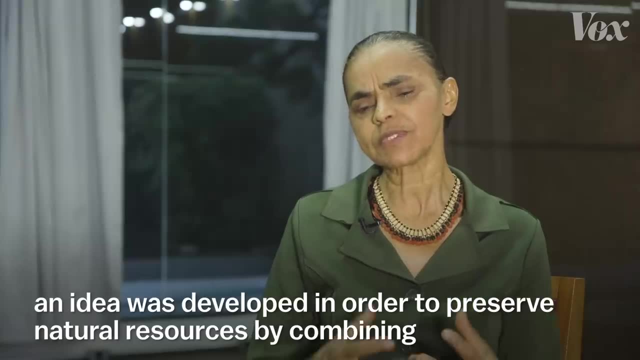 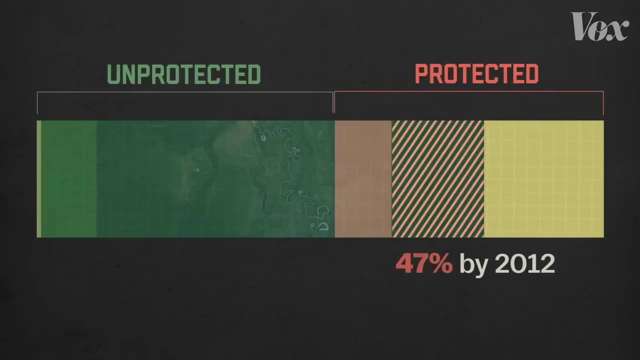 Based on this use and sustainable management, we began to think of a preservation and conservation idea of natural resources that would be able to integrate in the same equation economy and ecology. Eventually, almost half the Amazon would be put under some form of protection. 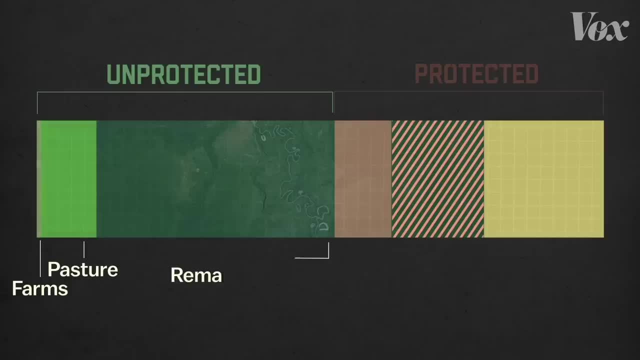 while the rest of it remained a mix of pasture farms and rainforests. To prevent further deforestation here the government strengthened the Forest Code, which said landowners could only clear 20% of their private land. This law was monitored by the Forest Service, which was part of the Environmental Ministry. 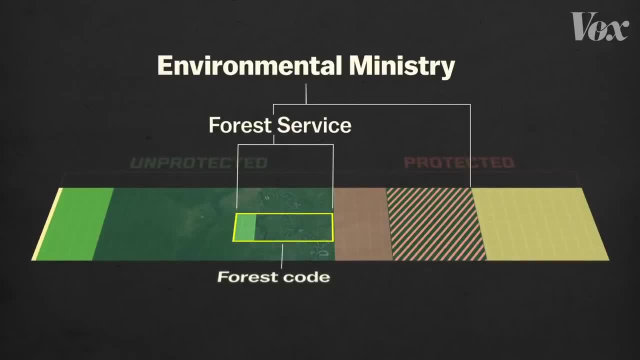 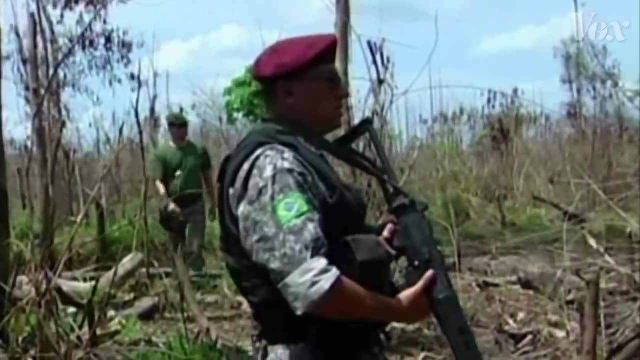 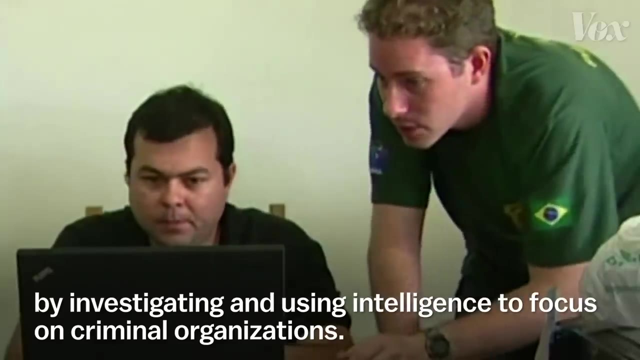 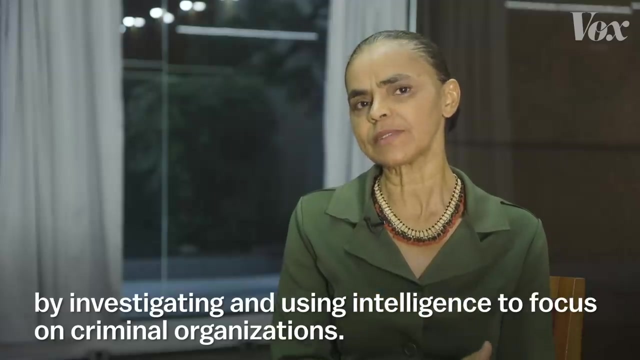 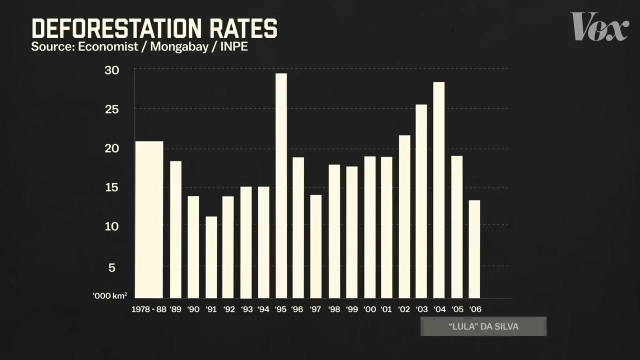 which had jurisdiction over all these protected lands, And the key to enforcing this entire plan was strengthening ABAMA, a police agency that would track and find people for illegal deforestation, And the plan showed results, with deforestation rates falling by more than half in 2006.. 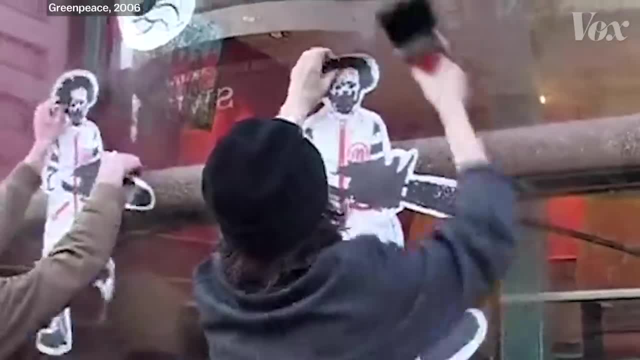 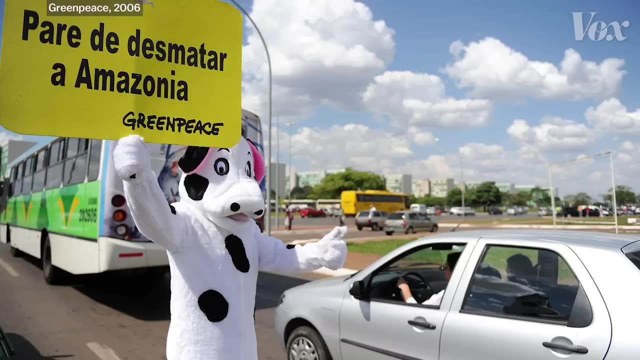 At the same time, an activist movement was forcing the agricultural industry to make a change. Major food companies started feeling pressure from consumers for participating in deforestation, So several got together and in 2006, signed a soy moratorium which meant they could continue. 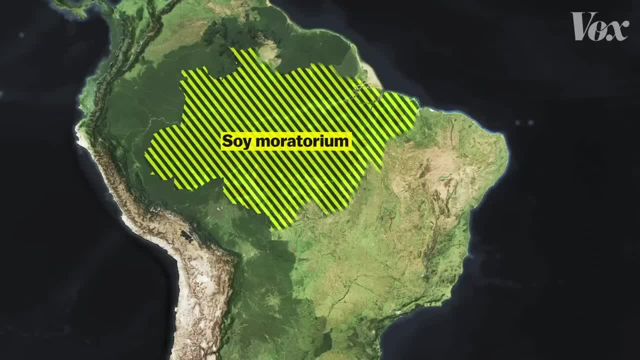 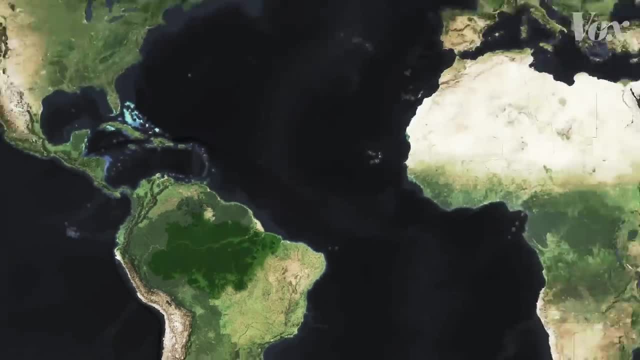 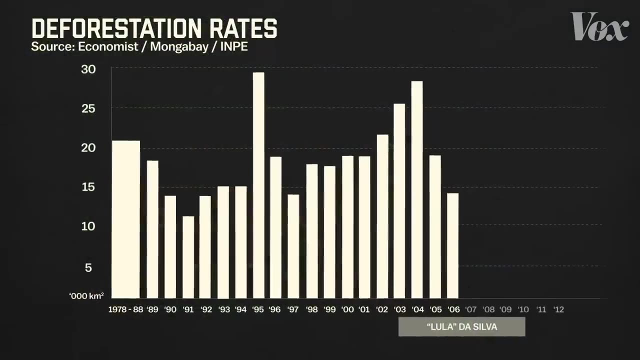 to operate within existing farms, but they wouldn't buy soy from any newly deforested land in the Amazon. Three years later, beef companies signed a similar agreement. Other countries also gave Brazil money to help it protect the Amazon. So under all this protection, deforestation rates plummeted to historic lows. 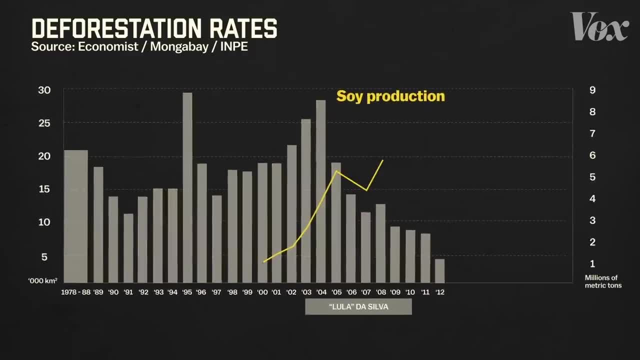 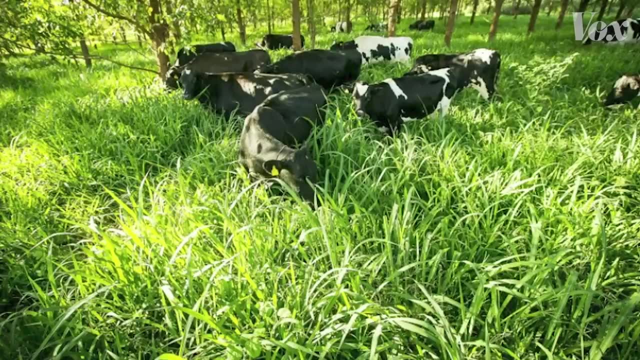 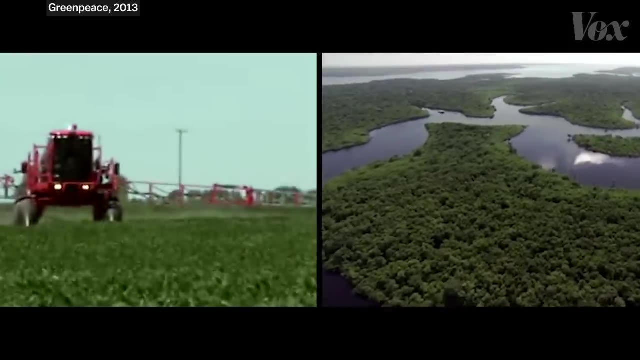 And yet Brazil's soy and beef industries continued to grow thanks to more efficient techniques. Ranchers started growing crops on their existing pastures, And farmers planted two crops a year on their land instead of one. Brazil had found a way to make the Amazon both productive and protected. 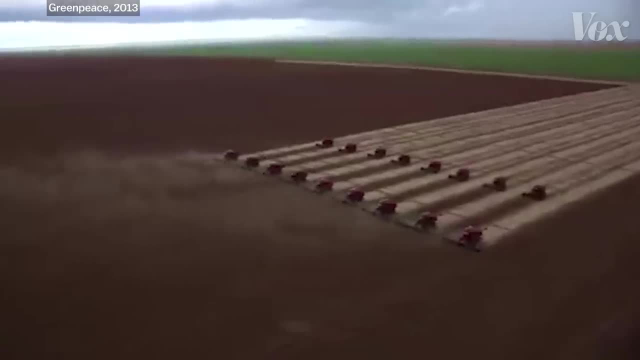 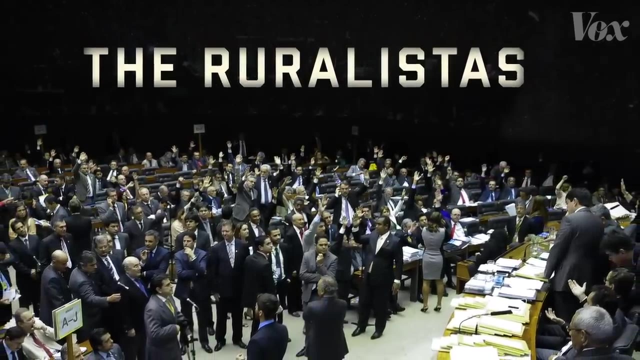 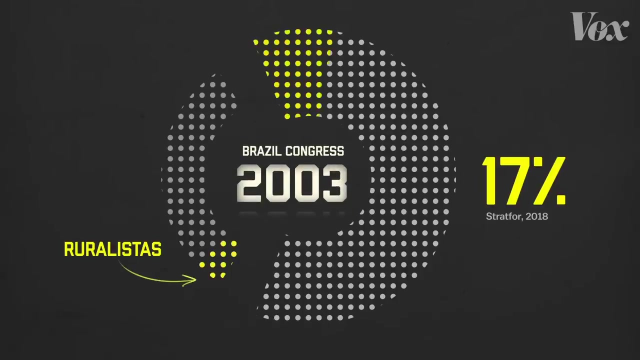 But there were some who still wanted it to be a more profitable place. The Ruralistas, a group of conservative politicians who represent the interests of the agricultural industry, including farmers and ranchers, started gaining influence in Brazil In the early 2000s. they had about 17% of the seats in Congress. 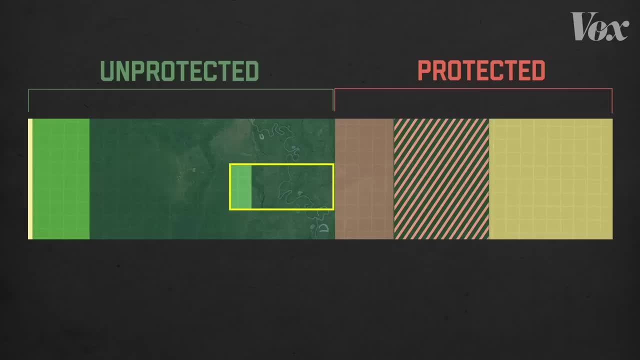 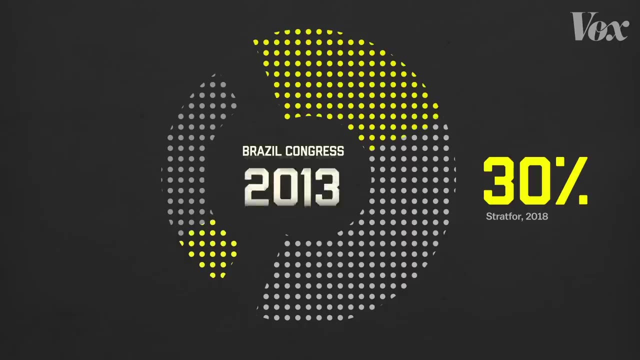 But by 2012, they had about 30% — enough power to push President Dilma Rousseff to weaken the forest code, which allowed landowners to get away with clearing more land. In 2016, they pushed President Michel Temer to slash Obama's budget. 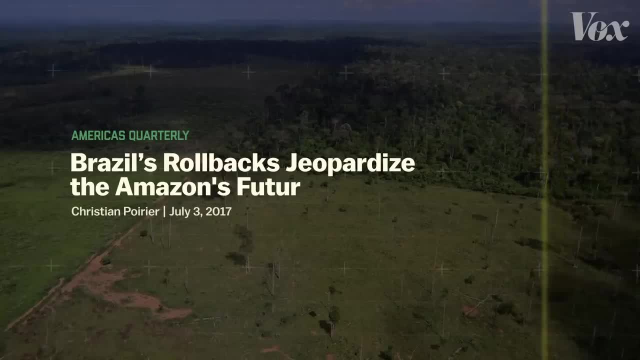 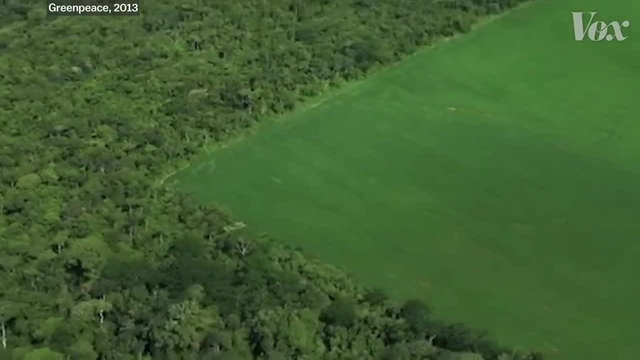 They also helped him pass a law that made it easier for people who illegally seized land in the Amazon to keep it. These changes emboldened some people to seize and clear the rainforest again, And that led to a rise in deforestation rates. 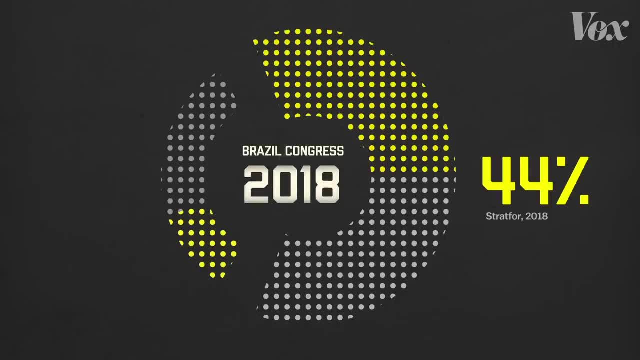 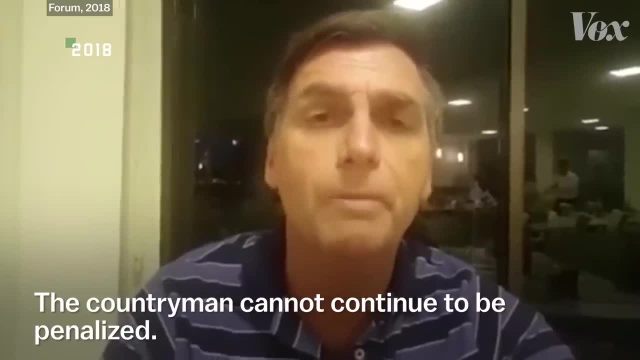 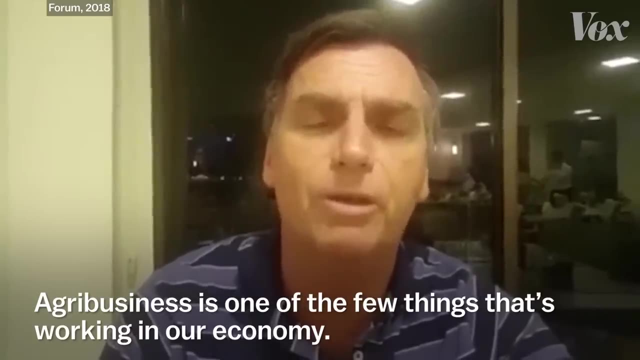 In 2018,, as the Ruralistas controlled 44% of Congress, Jair Bolsonaro, a right-wing congressman and ally to the Ruralistas, was elected president. The farmer cannot continue to be penalized. The agribusiness is one of the few things that is working in our economy. 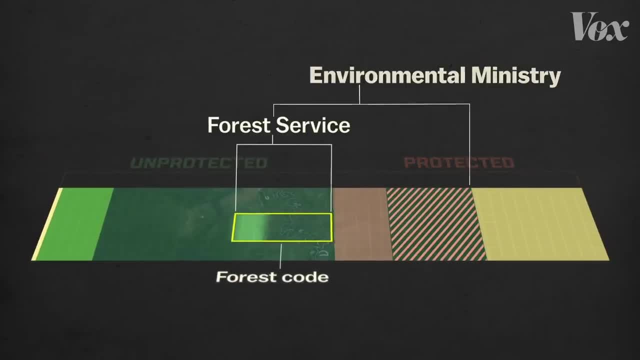 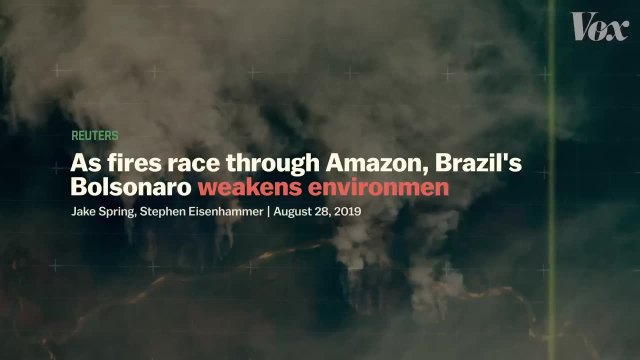 On his second day in office, he transferred the farm to the Ruralistas. He was the first person to be penalized. He transferred the Forest Service, which monitors the forest code, to the Agricultural Ministry. led by a Ruralista, He's also worked to systematically weaken the environmental ministry. 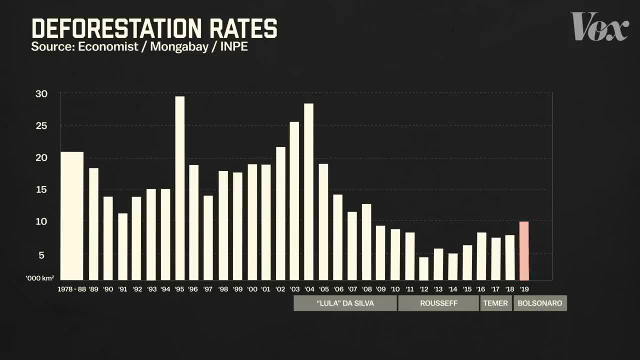 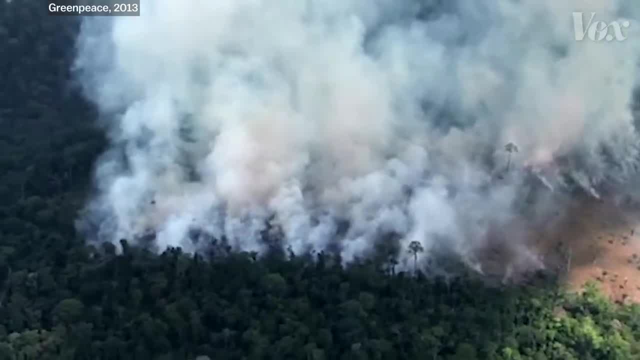 Under Bolsonaro, deforestation has increased significantly in 2019, most of it taking place in these protected areas. Setting fires is a common way to clear land, And in August 2019, over 30,000 fires were burning in the Amazon. 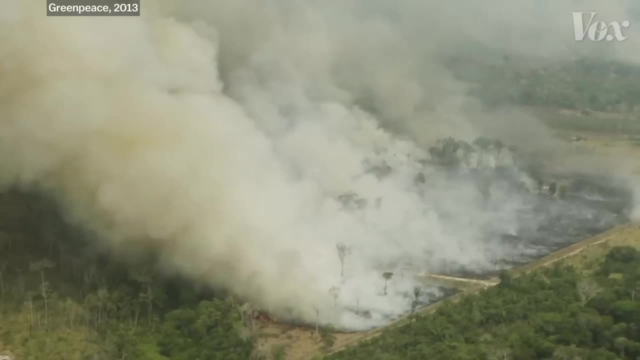 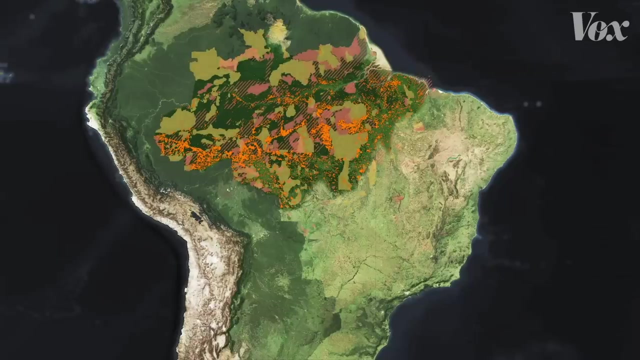 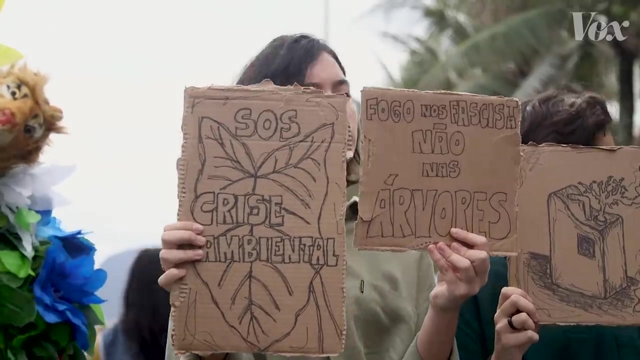 Three times as many as August 2018.. Many set illegally by ranchers, farmers and landowners, emboldened by the government's new stance on the Amazon. But this time the Amazon is unlikely to survive another wave of deforestation. In the last 50 years, it's estimated that about 17% of the Amazon has been deforested. A 2018 report estimated that if it reaches 20 to 25%, the whole Amazon would be deforested. The Amazon has been deforested. 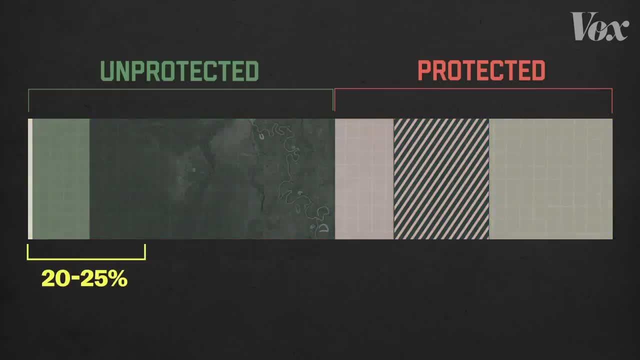 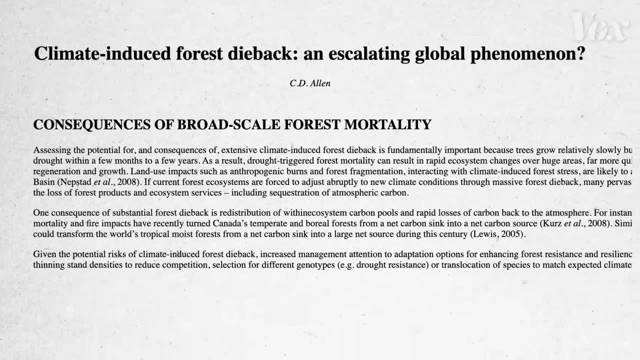 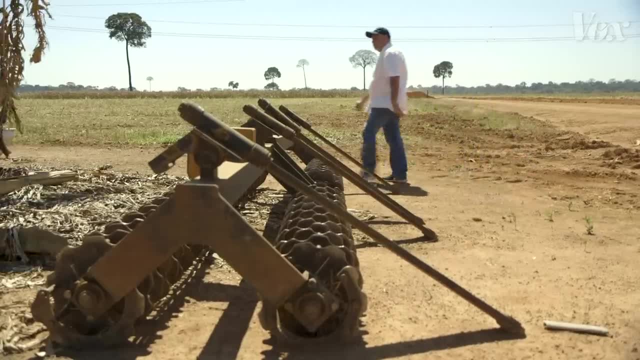 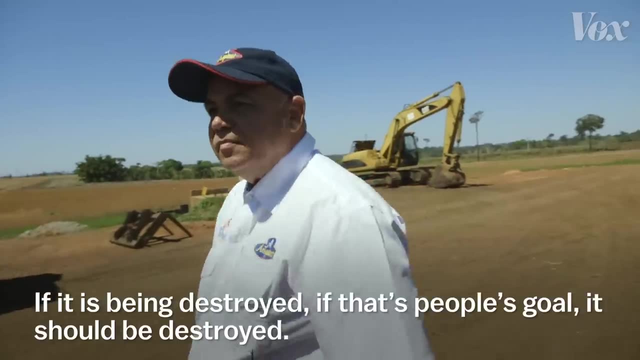 It wouldn't be enough to cycle all the water it needs, causing trees to die, And that would release a huge amount of carbon dioxide into the atmosphere, further warming the planet. But in Brazil, many politicians and agricultural businesses continue to ignore the science. 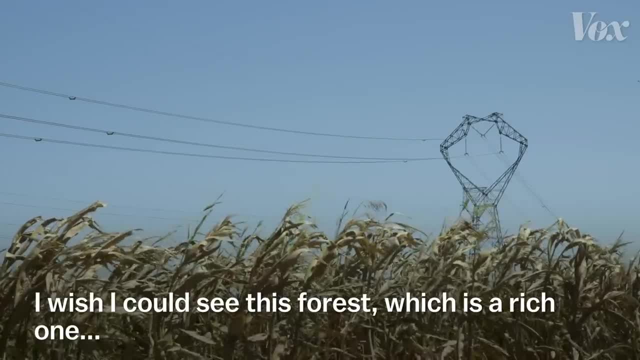 for the sake of profit. God knows what nature does If it's destroying. the goal of the world is to be destroyed, even because it's a very rich forest right. But my real desire was to see it the way I see it here in my farm. 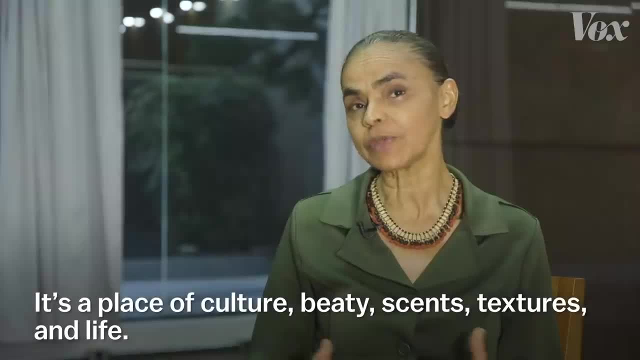 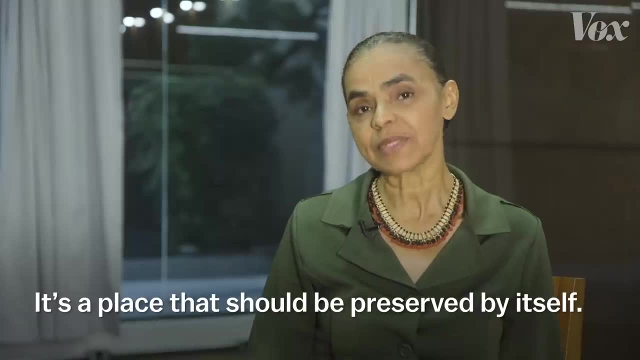 my property here. It's all on the ground. It's a place of culture, it's a place of beauty, it's a place of aromas, of textures, of life, So it's something that must be preserved. Clearing the Amazon for short-term gains.